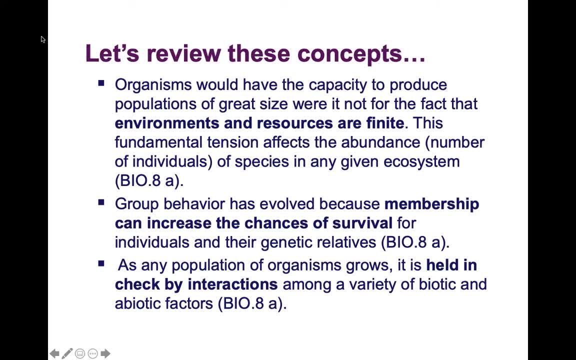 started. So let's start by reviewing these concepts first, and these are part of your standards and essential understandings. So organisms would have the capacity to produce populations of great size were it not for the fact that environments and resources are finite- This fundamental tension. 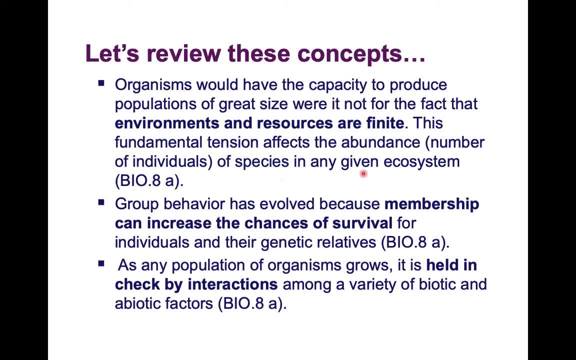 affects the abundance number of individuals, of species, in any given ecosystem. So this is pretty much saying that if it weren't for the limited resources and the finite resources, then populations would just grow out of the system. The next concept is group. behavior has evolved because membership can increase the chances of 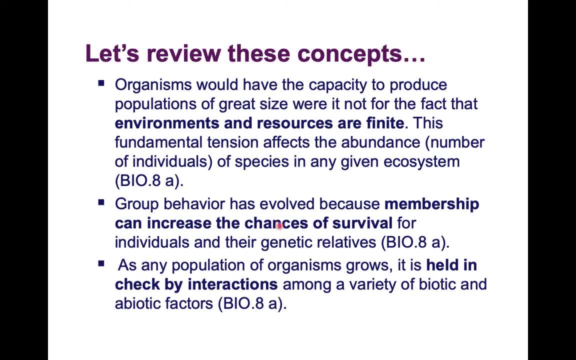 survival for individuals and their genetic relatives. So this just means that you're safer if you're part of a pack. if you're part of a group, That increases your chances of survival And any population of organism grows. It is held in check by interactions among a variety of biotic. 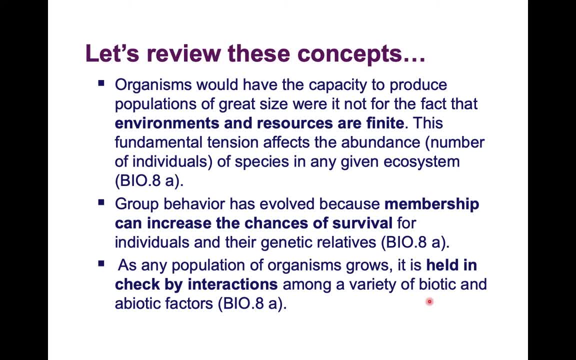 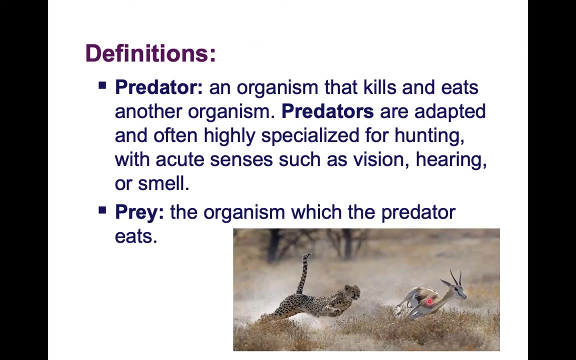 factors. So we talked a little bit about the limiting factors in the last lesson and how these limiting factors can affect how a population grows And it can affect that a population. it can limit the size of the population. So let's start with a couple of definitions and make sure you write. 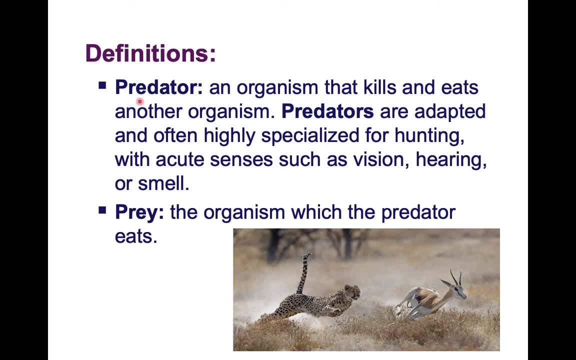 those definitions down in your note taker. So the first definition is the definition of a predator, And this is an organism that kills and eats another organism. So of course, the predator in this picture would be the cheetah, And they are adapted. 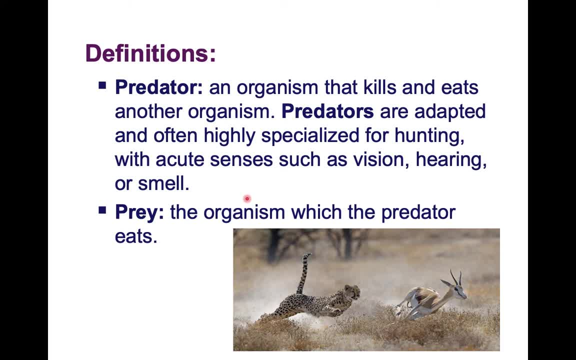 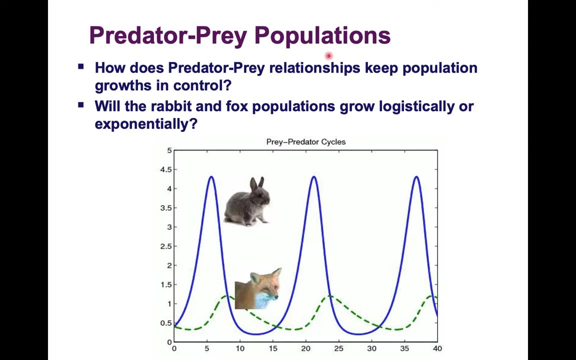 and often highly specialized for hunting, with acute senses such as vision, hearing or smell. And then the prey: the gazelle is the organism which the predator eats. So let's look at the definition of a predator, predator-prey populations, and let's look at this graph. and while we explore this, 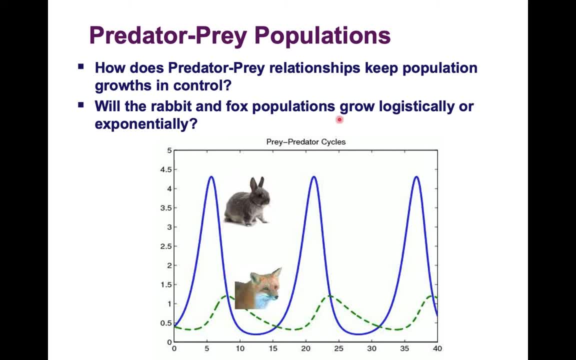 graph. see if you can answer these two questions on in your note taker. so the first question is: how does predator-prey relationships keep population growths in control? so what do you see happening here? so here we see the rabbit population is going up and down, up and down, up and down, so it is fluctuating. 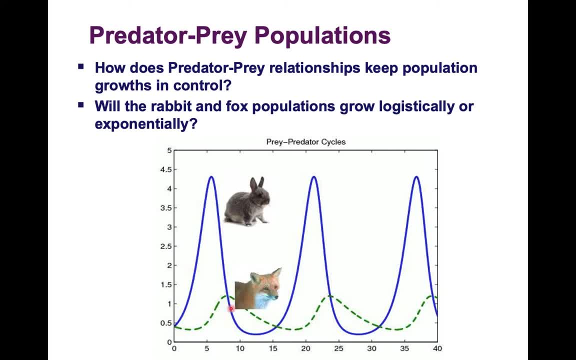 around its carrying capacity at a steady state. and then we see the same thing with the fox population. right, it's also going up and down, up and down, up and down. now, the first thing that you might notice here is that the prey population is a lot larger than the predator population. 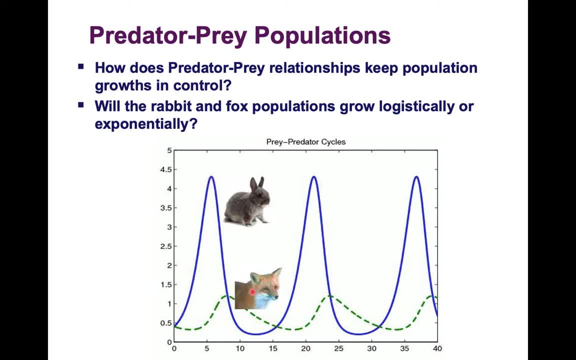 so there is usually more preys out there than predators. okay, so as the prey numbers go up, right, what do you see happening to the predator numbers? well, they go up too right. so there's a lot of food to eat, so the predator number goes up. so what happens, or what triggers the prey population to start going down? 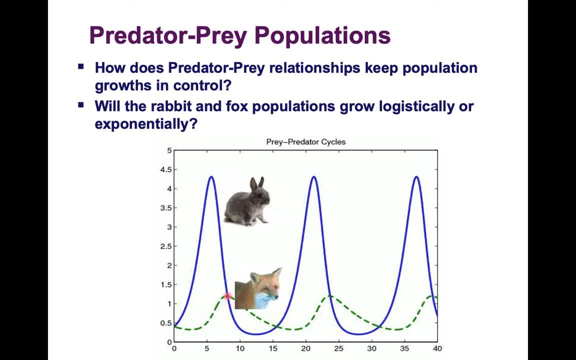 well, probably that there's too many predators out there, right? so there's a lot of predators and they feed on a lot of prey, so that causes the prey numbers to go down. okay, so notice how they're controlling each other. see, as the prey population goes up, so does the predator population. right now there's a lot of. 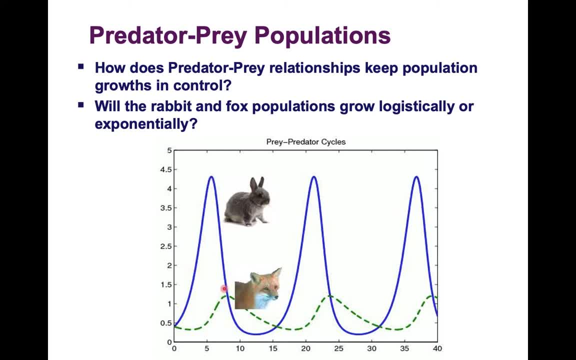 prey, but there's also a lot of predators. so that means that these predators are going to be controlling each other. so that means that these predators are going to eat a lot of prey, which means that the prey number starts to go down. and as the prey number starts to go down, what happens to the predator number? it also 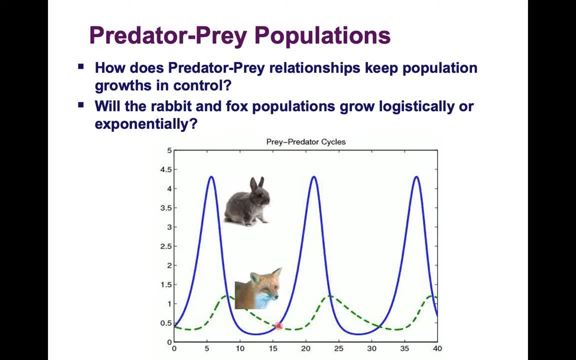 starts to go down right. so these populations are controlling each other in a good way, right? you don't want this prey to grow out of control and you don't want this predator number to grow out of control. so these predator prey populations and interactions are actually good interactions. we need them. 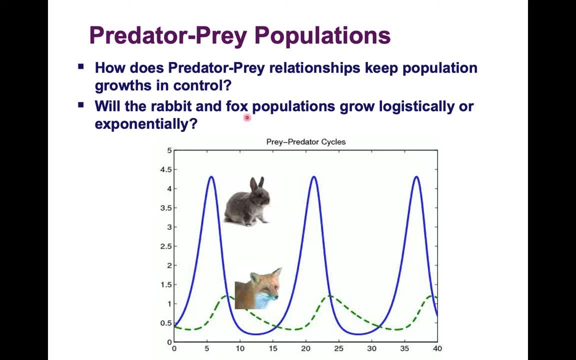 as part of a healthy ecosystem. so then, to answer the next question: will the rabbit and fox populations grow logistically or exponentially? so, do you see a J curve here? well, initially right, but then what's going to happen? they're going to fluctuate around their steady state and then they're gonna drop, and 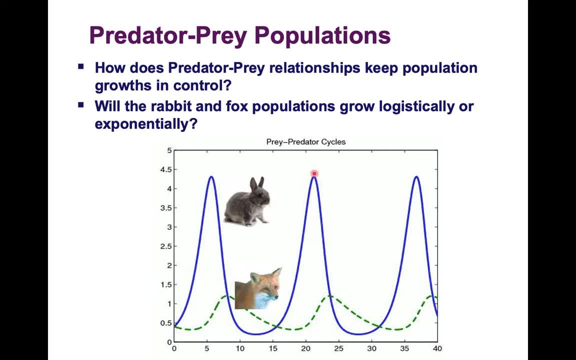 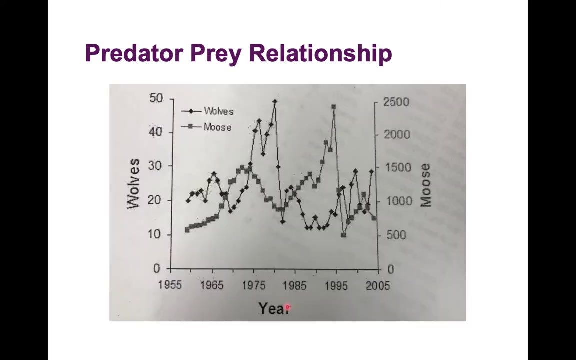 then they're gonna go back up. so we see a logistic, balanced growth. right, because they are just not growing exponentially out of control. there is a control of their growth, both their growth. so both populations are growing logistically. so here we have another example of a predator prey relationship: the wolves and the moose population. so here, as you, 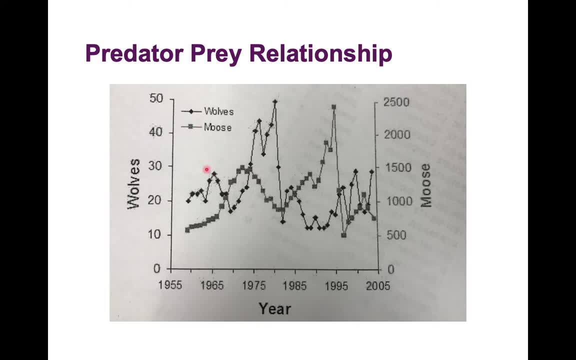 explore this graph, you see the same thing is happening, right. so here we see the moose population. it starts to go up and then, because there's a lot of moose, meaning there's a lot of food for the wolves, we also see the wolf population start to go. 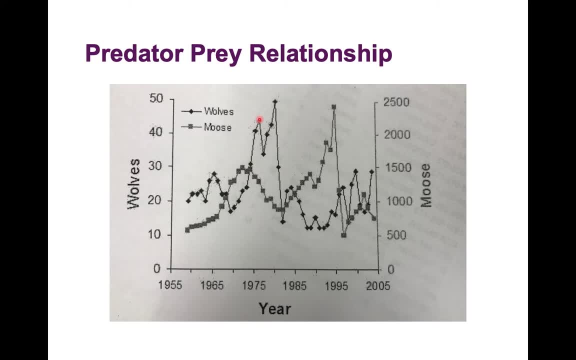 up right, but now there's too many wolves out there preying on the moose, which means that the moose population is going to start to decrease and now there's a very little food for the wolves. and you see, the wolves look a lot better than before in dis zadashok. wolf population starts to go up. more biofi makes up all of the pretty big queens. now we have very little food for the wolves, for the wolves, and you see the wolves are getting schooled very quickly because bulls must kem experiment a lot more frequently just to get big supplies that walk off of the south. well, in 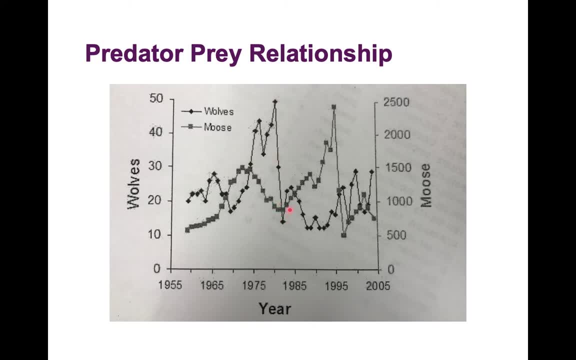 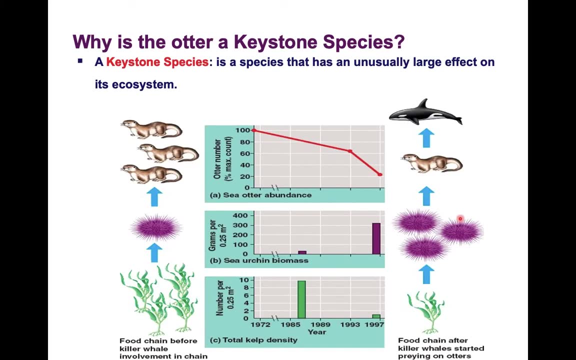 see the wolf population starting to go down right, And then it's a cycle that repeats itself throughout the years. All right, moving on. So let's explore the term keystone species And let's try to figure out here why is the otter a keystone species? So the definition of 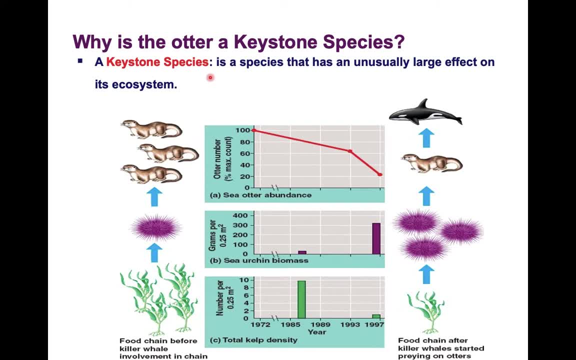 a keystone species that you're going to need to write down in your note taker is that it's a species that has an unusually large effect on its ecosystem. So let's see what's happening here. Let's look at this food chain. Oops, let's look at this food chain here before the killer whale. 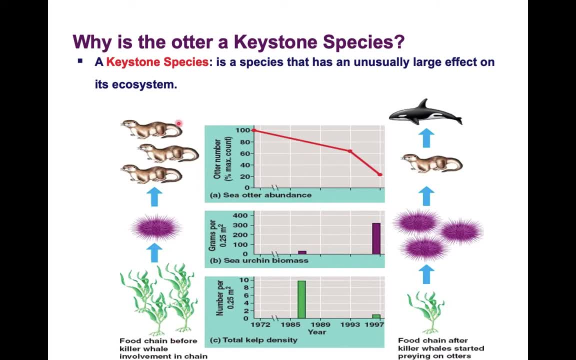 was introduced. So here you see the sea otter abundance, which is at about 100%. Okay, Around this time you see that the sea urchin abundance. it's around, you know, somewhere around. I don't know about a hundred percent, So it's around a hundred percent. 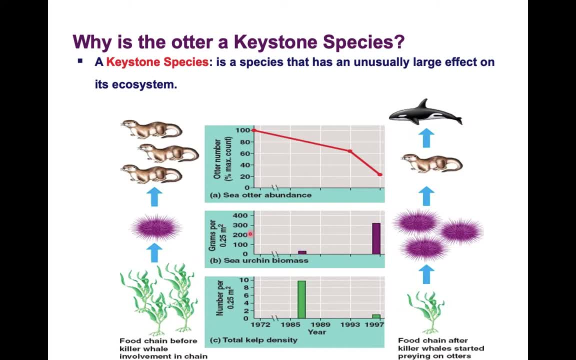 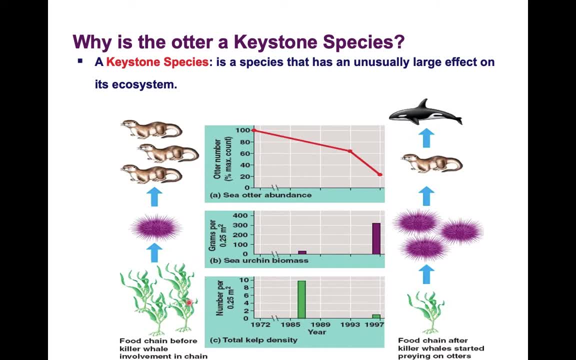 per meter square And you see, the kelp density also is pretty high, right Around 10 per 0.25 meters squared. So what happens when you introduce the killer whale into this ecosystem? So as you introduce the killer whale, what happens? 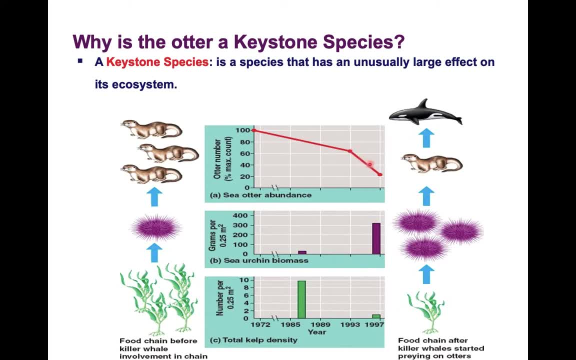 What happens to the otter population? The otter population starts to go down. Notice that it's decreasing, right As you decrease the otter population. what happens to the sea urchin biomass? Well, that starts to go up. And then what happens to the kelp density? So kelp is 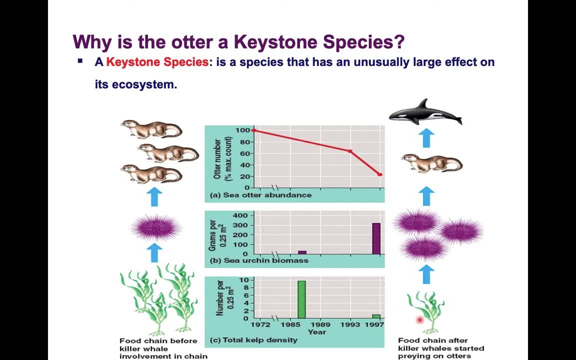 an aquatic plant that grows in the bottom of ocean floors. So you see, the kelp is decreasing. Actually, kelp is not a plant, It's an algae, if you want to be more specific. But anyways, the kelp population is decreasing. So what did the killer whale introduction do to this? 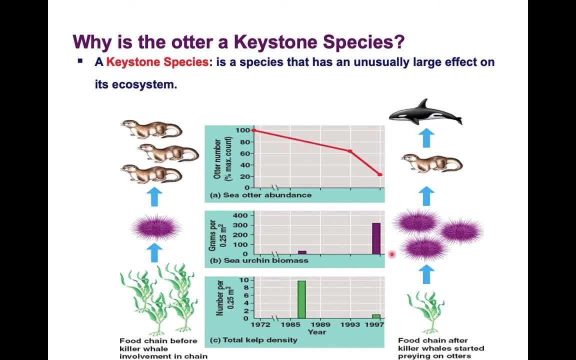 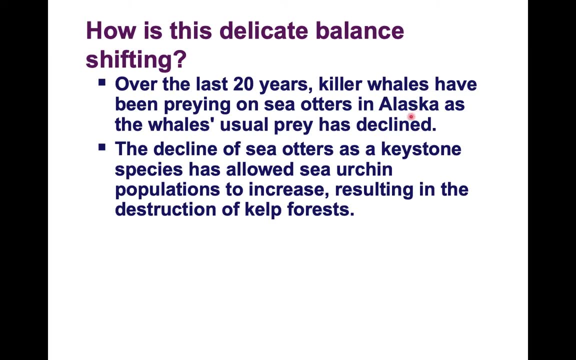 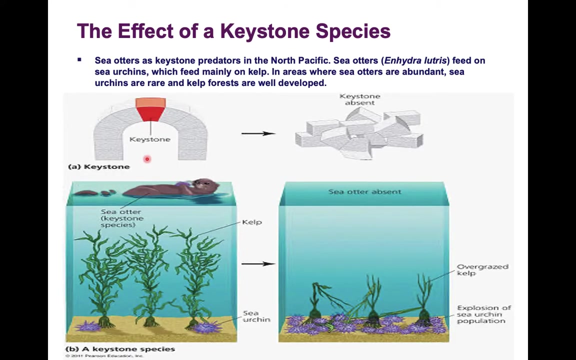 ecosystem. Do you think it had an effect when this killer whale was introduced? So let's look at this delicate balance. So let's look at this delicate balance. So let's look at this delicate balance. So, over the last 20 years, killer whales have been preying on sea otters in Alaska, as the whale's usual prey has declined. The decline of sea otters as a keystone species has allowed sea urchin populations to increase, resulting in the destruction of kelp forests. So here are the sea otters. Pretty cute, right? The sea otters are a keystone species And what they do is they 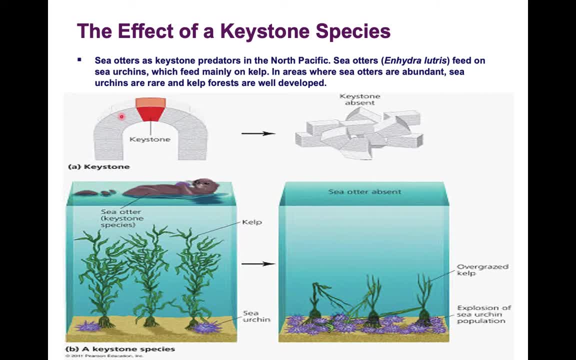 hold this ecosystem in the North Pacific intact and in place, That keystone species here. it's a very important piece of the ecosystem that if it's missing, if it's absent, the ecosystem kind of collapse. So this keystone species, the sea otter, it feeds on the sea urchins right And the sea urchins feed on the kelp. So you want to have a healthy amount of kelp. 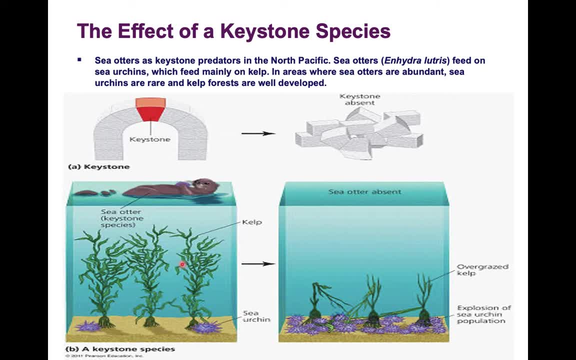 in the ocean floors. right, Because they provide a habitat for other organisms. But what happens if the sea otter is absent? Then you're going to have an explosion of sea urchin populations and they're going to overgraze the kelp and it's going to destroy this habitat. So the sea otter is a very 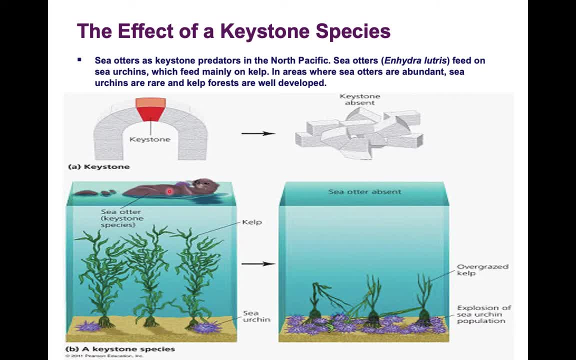 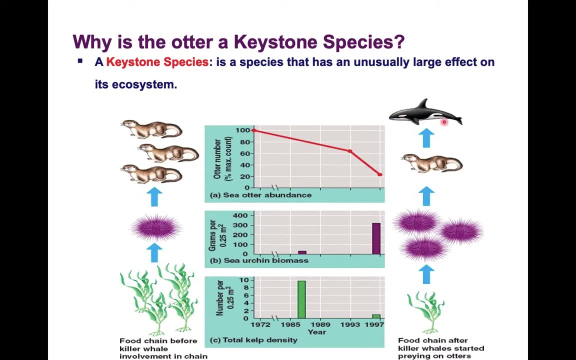 important species known as a keystone species, and you want them to be there, But we just learned that, as the killer whales are being introduced into these ecosystems, they are feeding on the sea otters and killing them, which means that the sea urchin biomass increases, which means that 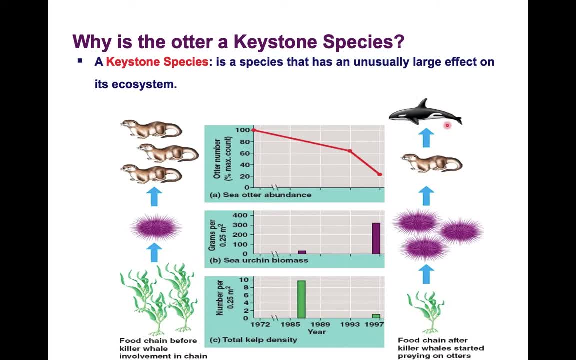 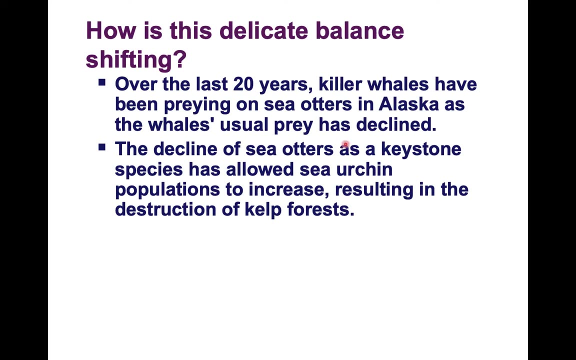 there's overgrazing of kelp. So this killer whale introduction is not a good thing, right? Because you are destroying that keystone species that is actually needed. So who is introducing killer whales into areas in Alaska where they shouldn't be going? Well, 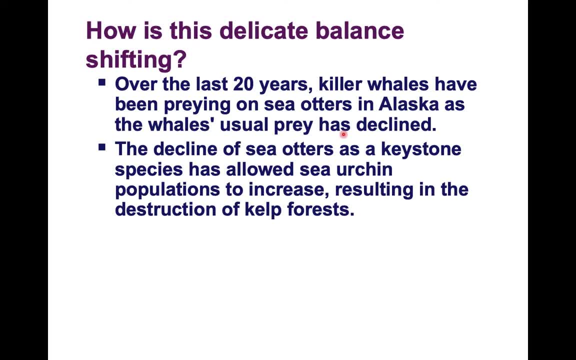 of course it's humans right. So as humans destroy the habitat of whales and because of humans preying on whales and destroying the food and prey of whales, these killer whales are going to be in the sea. So who is introducing killer whales into areas in Alaska? 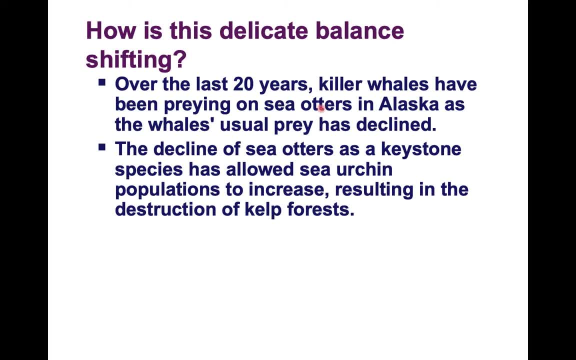 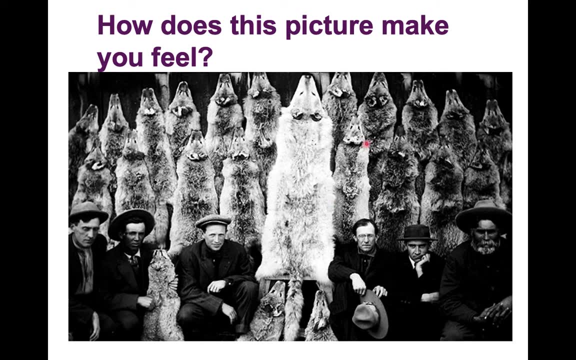 whales have had to move into areas where there are sea otters, and then these killer whales are now destroying the sea otters and ruining this delicate ecosystem. So, besides how humans have affected the keystone species known as the otters in the Alaskan ecosystem, how else have humans 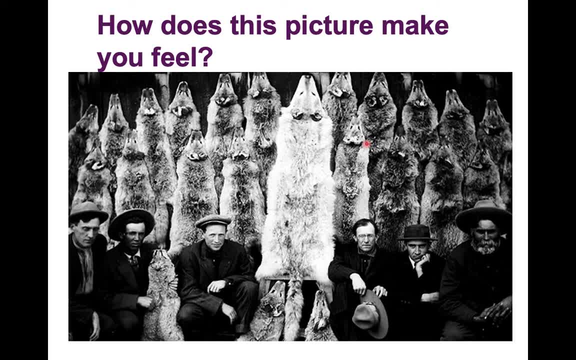 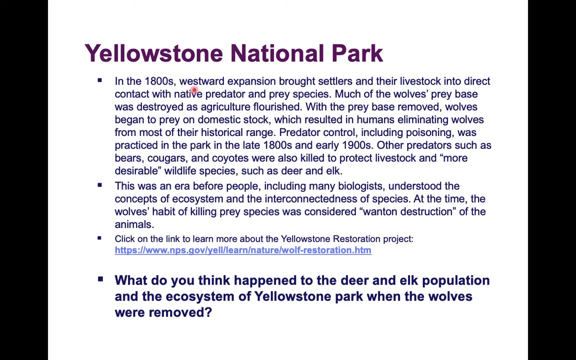 interfered with other keystone species. So how does this picture make you feel? What do you see here? You see wolves, right, You see dead wolves as they were being hunted by humans. So a little background on this picture. In the 1800s, westward expansion brought 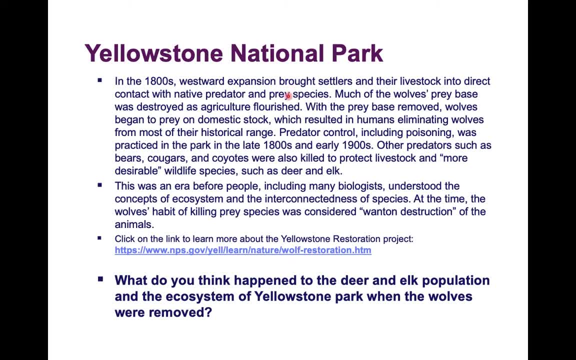 settlers and their livestock into direct contact with native predators and prey species. Much of the wolves' prey base was destroyed as agriculture flourished. With the prey base removed, wolves began to prey on domestic stock, which resulted in humans eliminating wolves from most of the 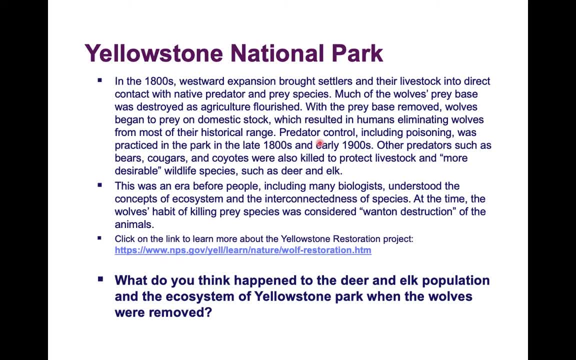 historical range. Predator control, including poisoning, was practiced in Yellowstone National Park in the late 1800s and early 1900s. Other predators such as bears, cougars and coyotes were also killed to protect livestock and more desirable wildlife species such as deer and elk. So this was an era before. 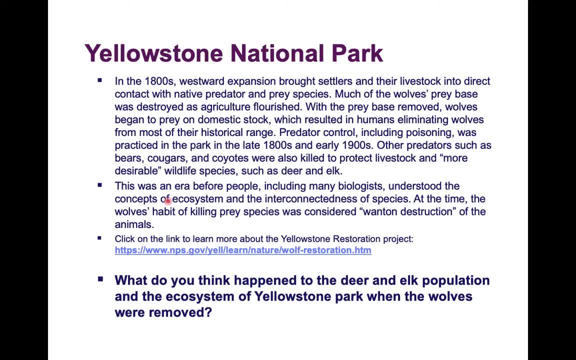 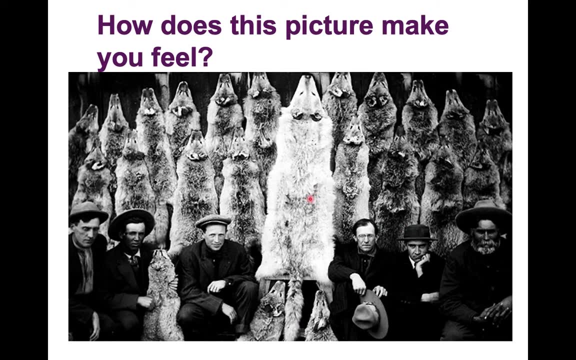 people, including many biologists, understood the concepts of ecosystems and the interconnectedness of species. At the time, the wolves' habitat of killing prey species was considered wanton destruction of the animals. So here in this picture we see that in a time where 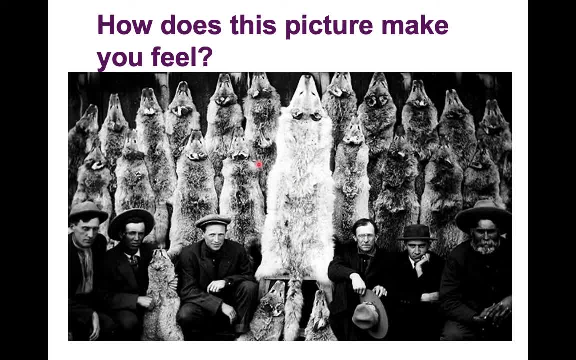 it was actually encouraged for people to hunt these wolves in Yellowstone National Park Because, as you just heard, these wolves were preying on the domestic livestock And of course that was not a good thing for the farmers. The reason why the wolves 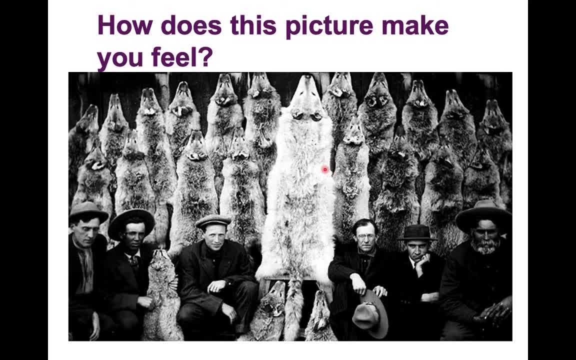 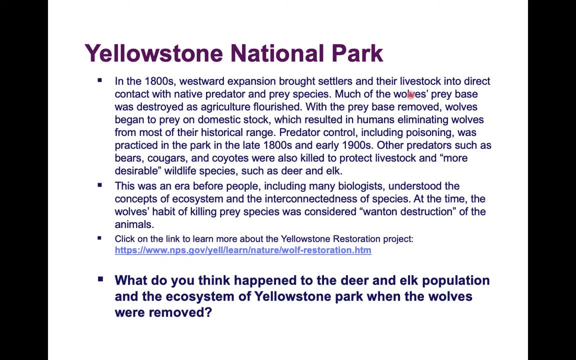 had to go and prey on the domestic livestock of farmers is because humans pretty much settled and came into direct contact with the habitat of these wolves and the natural prey of these wolves. So these wolves had no other place to go right And they had no other prey to. 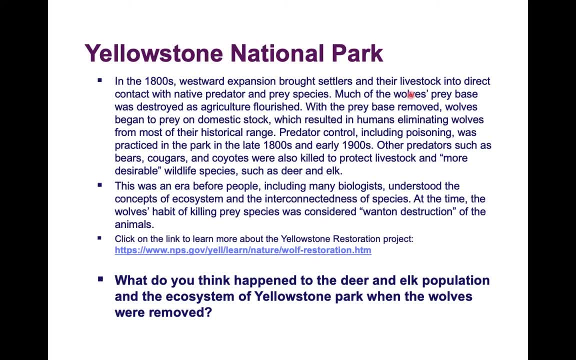 feed on other than the domestic stock of humans. So if you want to learn a little bit more about the Yellowstone Restoration Project, you can click on this link and this will tell you. well, what did we do right Or what happened? So we destroyed, pretty much decimated. 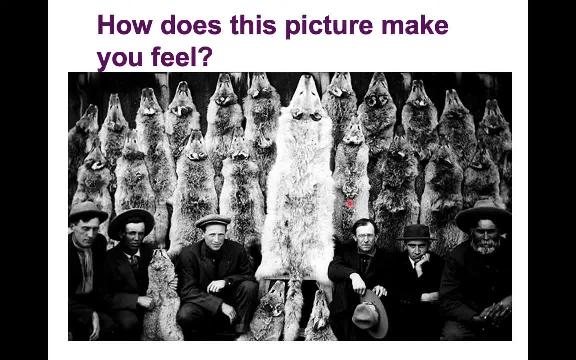 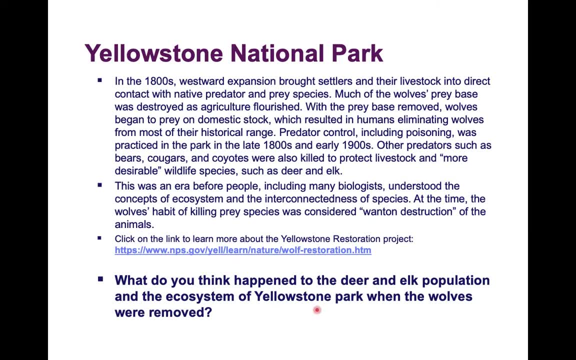 the wolf population in Yellowstone National Park. So what was done to restore the wolf population And what do you think happened to the deer and elk population and the ecosystem of Yellowstone Park when the wolves were removed? So here is a picture of the before and after. 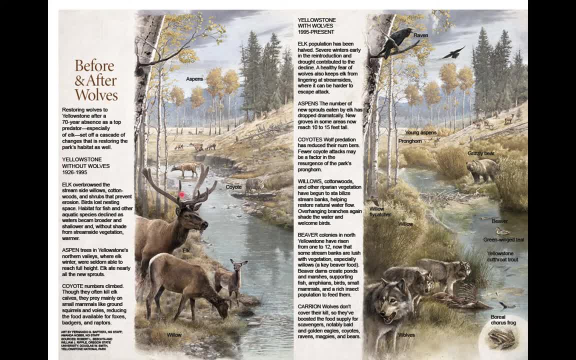 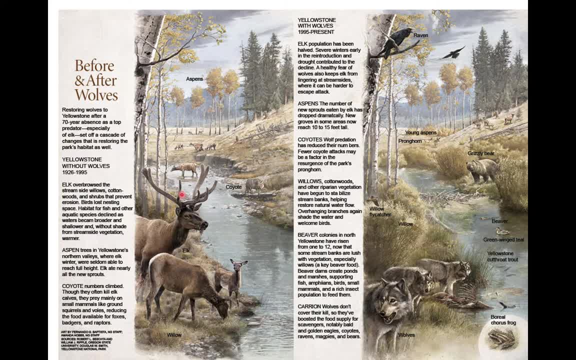 are a keystone species. And now how the wolves are a keystone species. So notice what happened to the Yellowstone National Park when there was a 70-year absence of the wolves as a top predator. So the elk overbrows the streamside willows. They pretty much destroyed the aspen trees. 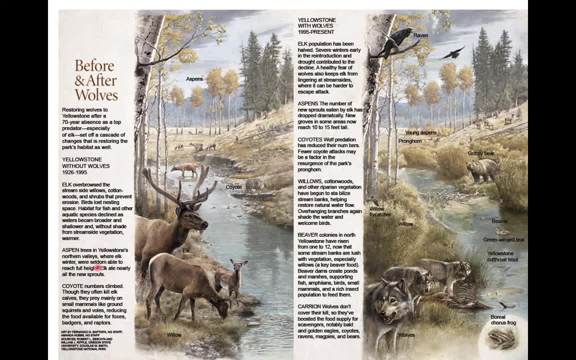 The trees were seldom able to reach full height, as the elk ate nearly all of the new sprouts. Because there was a loss of trees, then that means that other habitats were also destroyed- Side willows, cottonwoods and shrubs that prevent erosion- which meant that birds lost their 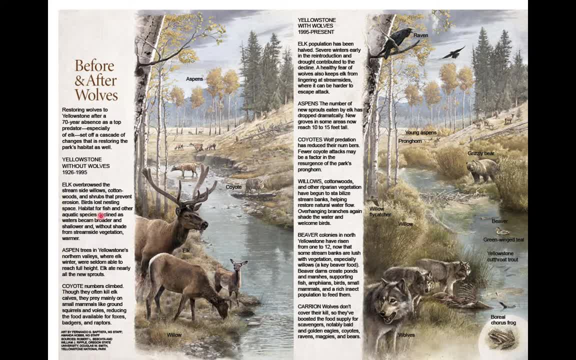 nesting space meant that habitat for fish and other aquatic species declined as waters became broader and shallower and without shade for a streamside vegetation, they also warmer, and the coyote numbers climbed. though they often kill elk, calves, they prey mainly on small mammals like ground squirrels and voles. reducing the 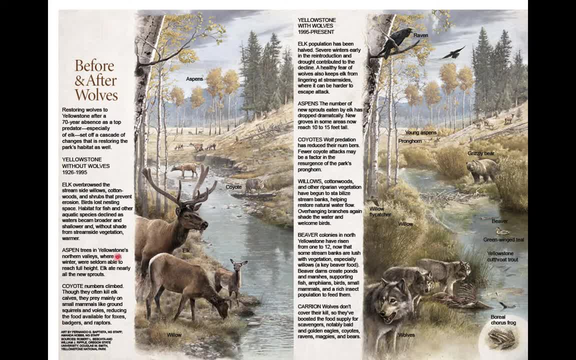 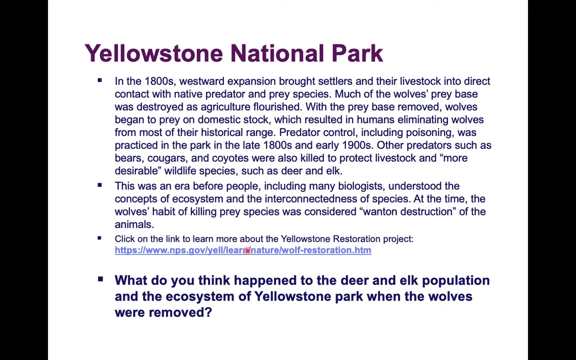 food available for foxes, badgers and raptors. so, as you can see from this picture, without the keystone species, without the wolves, the Yellowstone National Park East ecosystem was on the verge of collapsing. so, um there, like I said, make sure you you click on this link to learn about the restoration. 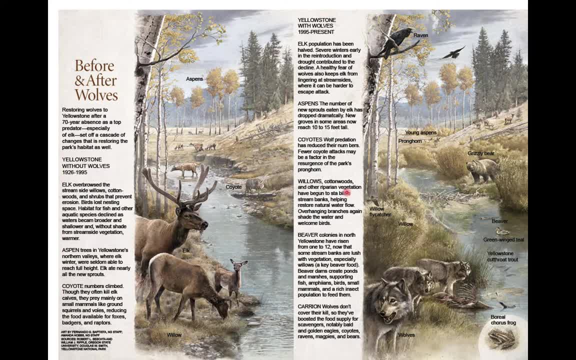 project. but wolves were reintroduced, reintroduced to the national park and they were reintroduced to the national park. but wolves were reintroduced to the national park and they were reintroduced to the national park and they were reintroduced to the national park and they were reintroduced to the national park. and when they were reintroduced we saw 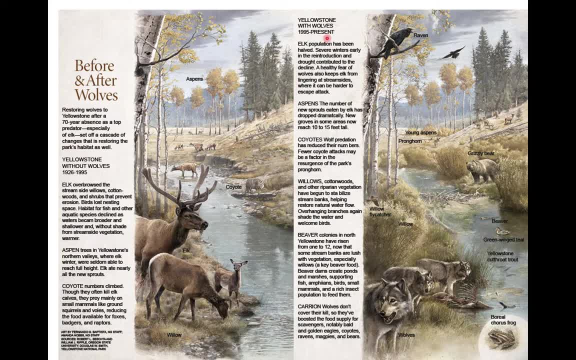 reintroduced to the national park and when they were reintroduced we saw reintroduced to the national park and when they were reintroduced we saw what happened to the ecosystem from when they were reintroduced. we saw what happened to the ecosystem from when they were reintroduced. we saw what happened to the ecosystem from 1995 to present. so the elk. what happened to the ecosystem from 1995 to present, so the elk. what happened to the ecosystem from 1995 to present? so the elk population was halfed and that's a. 1995 to present, so the elk population was halfed and that's a. 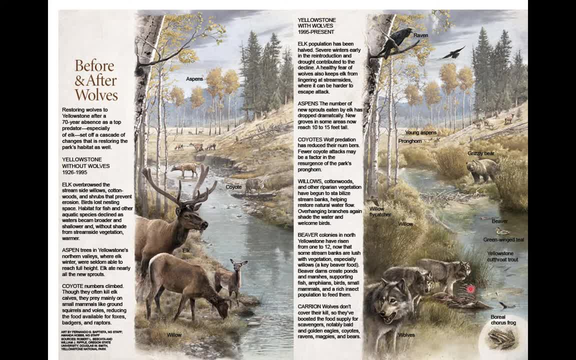 1995 to present. so the elk population was halfed and that's a good thing, right, because the wolves were population was halfed and that's a good thing, right, because the wolves were able to prey on the elk population. so that balance predator prey relationship was restored. 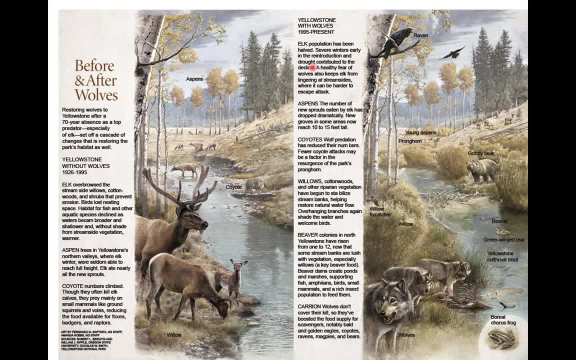 and as the elk population was halved, we'd see that the aspen trees started to sprout again. we start to see new groves in some areas. the coyote population was also reduced because of wolf predation, and then we saw willows, cottonwoods and other riparian vegetation have 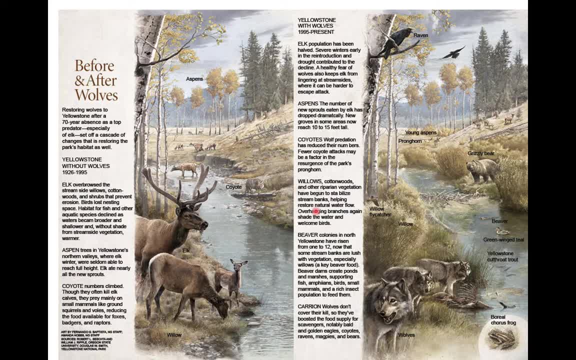 begun to stabilize stream banks, helping restore national water flow. overhanging branch branches again shade the water and welcome birds. beavers were back because now they had enough vegetation to build their dams. beaver colonies, um, it says here, that were, um they were able to um now rise, and you know, because of their lush vegetation. 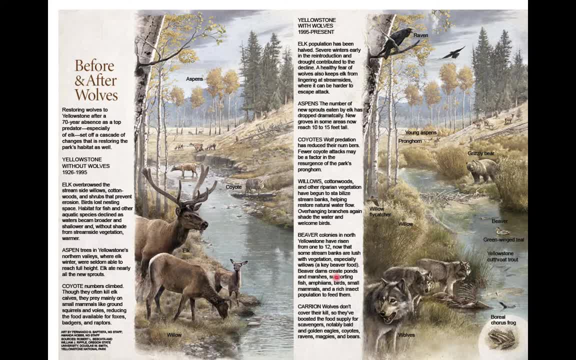 and now, with the beaver dams, they were able to create ponds and marshes supporting fish amphibians, birds, small mammals and rich insects populations to feed them and um and and another thing that happened here was that the beaver dams were able to create ponds and marshes supporting fish amphibians.